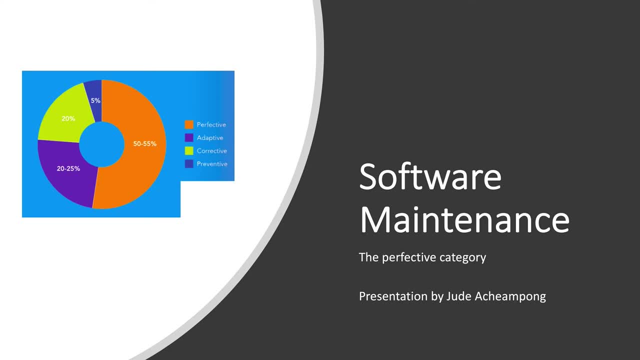 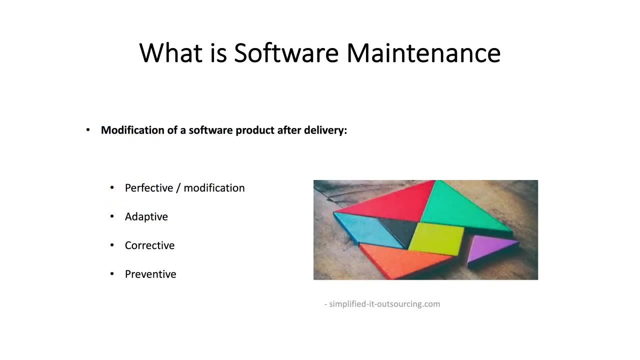 Hello, this is Jude, and today I will be presenting a video on modification or perfective category under software maintenance. What is software maintenance? The lifecycle of a software product never ends after the software is delivered to the customer. There is always a need to modify a software product for the purpose of perfective maintenance. 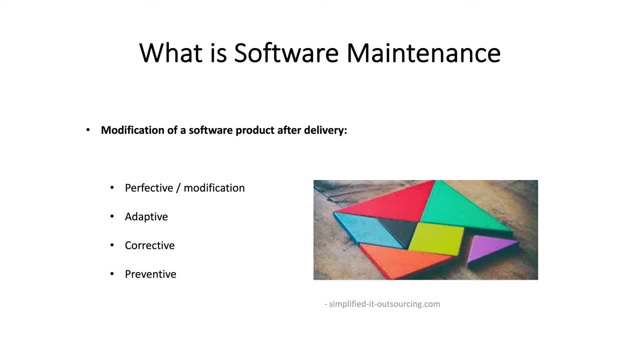 which improves performance. adaptive, which keeps a software usable in a changed environment. corrective, which corrects discovered problems. and preventive maintenance, which corrects faults. So hostel are the key tools to egg down the software complexity. The reason is, software is always evolving. 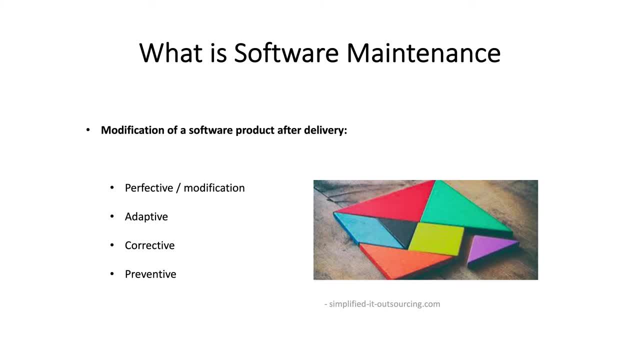 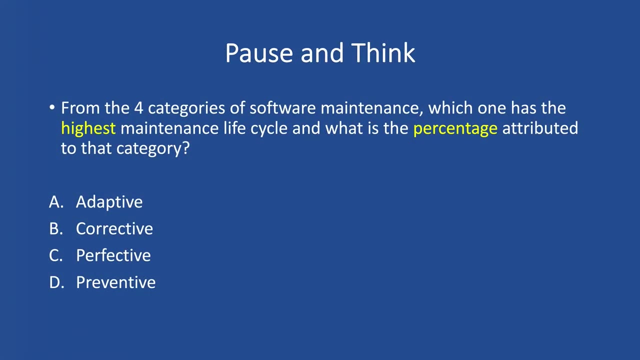 I will dive deeper into one of the categories of maintenance. First, lets test your knowledge of software maintenance, Jimmy, why do you put software maintenance in your esports coaching job? Well, the equation- psychologists provide us with the most basic understanding of software maintenance- is that when many golfers mask one ball based on the shape of the stock it holds, the 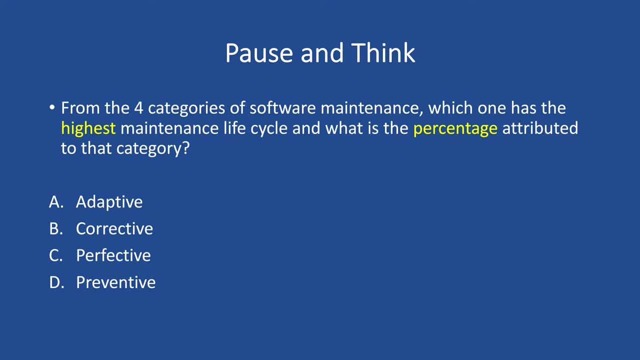 top of that ball maintenance, Which one has the highest maintenance lifecycle And what is the percentage attributed to that category? Please pause the video and try to figure out the category. I will give you 10 seconds to do that. Okay, I hope you were able to get the answer. 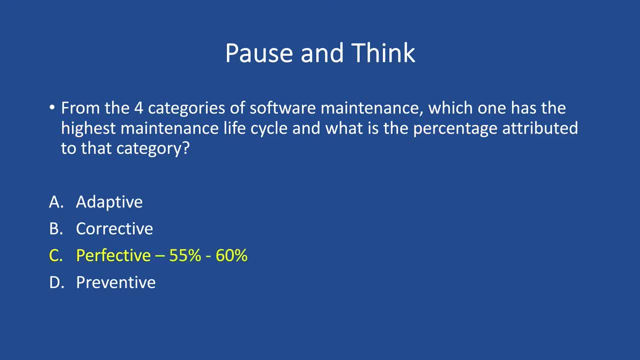 Perfective maintenance. There is a constant request to modify software products after delivery to improve performance or maintainability. The reason is: as users get exposed to the software, there is a need for new features. Interestingly, studies suggest perfective maintenance makes up 55 to 60 percent of. 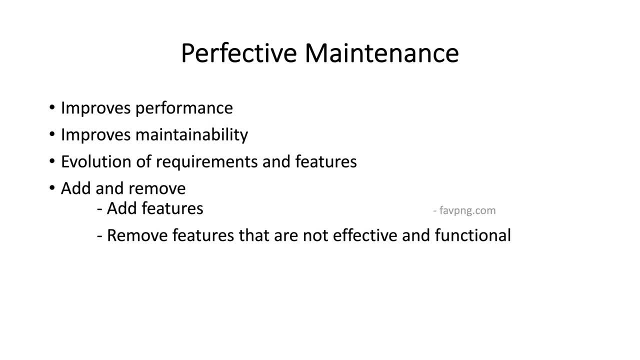 software maintenance. Before I go over perfective maintenance, it's important to mention that software maintenance is more than just bug fixing. As the software is being used and exposed to the ever-changing technology world, there will be a reason for perfective maintenance. Users may. 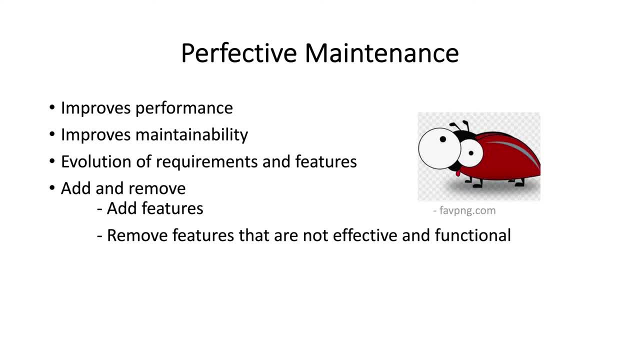 experience poor performance. When this happens, there's a need to improve performance. Furthermore, when there is a need for an efficient software management, there is a a request for developers to improve the software. for maintainability, Suppose there is a need for new features to be added to the software. 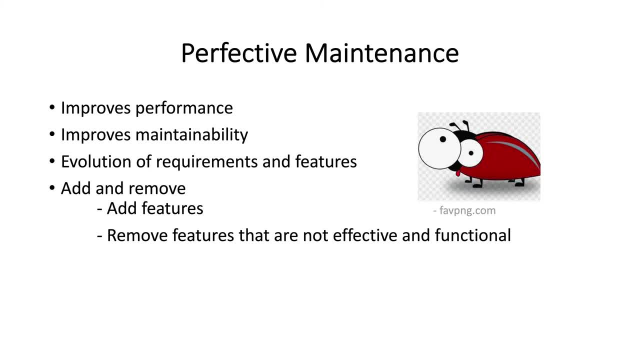 Then perfective maintenance plays a role in the evolution of requirements and adding features. Also important is removing features that cause a software to not be effective or function properly. Whatever the motivation is for maintenance, perfective maintenance is important and will always be a key to a successful software. 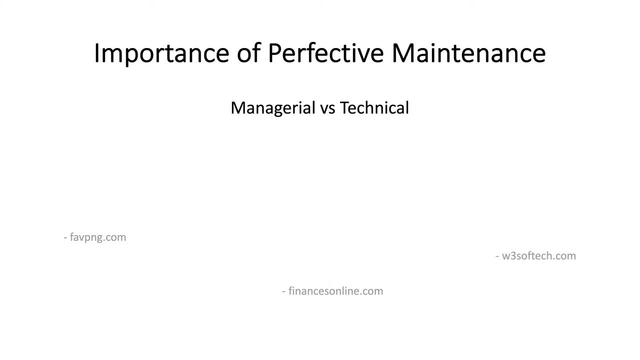 There are reasons for, and importance of, perfective maintenance. These reasons and importance are both managerial and technical. Managerial issues include customer priorities. As customers use the software, the requirements might change. There needs to be a balance to be made In order to meet customers' needs. 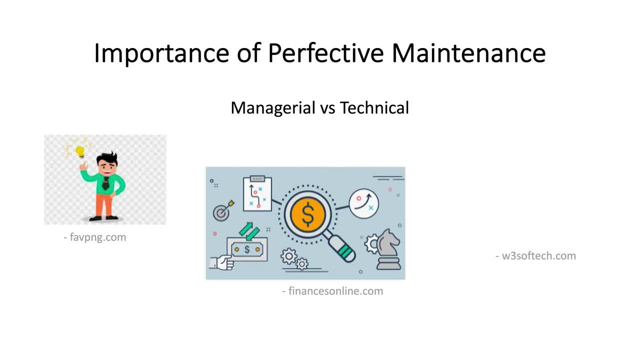 Estimating cost is a managerial responsibility and there is always a need to enhance the software to reduce cost. On the technical side, testing is vital to a software product. Developers must test. Developers must test, test to perfect a software and to add functionalities for maintainability measurement. 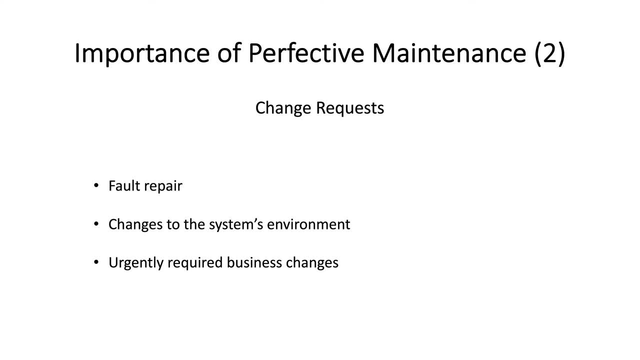 In addition to the importance and reason for perfected maintenance, there are continuous change requests sent back to maintenance developers. Some of the change requests are fault repair. these could be bugs. Another request is software must also consider the system environment and changes must be made to fit that environment. 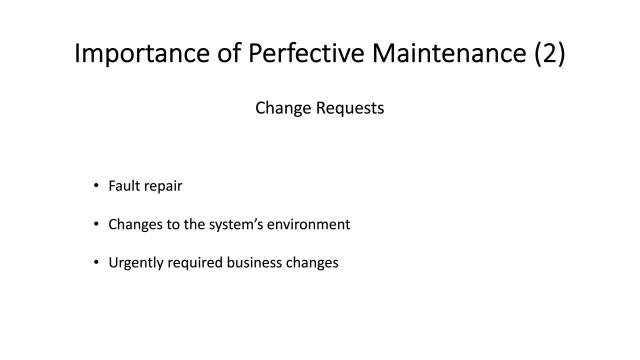 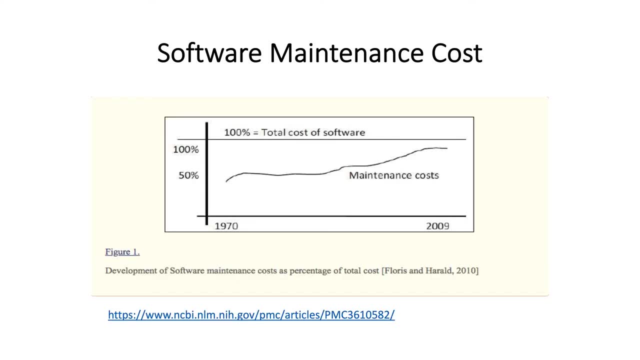 Also business changes like functionality can also contribute to change requests. It is not a surprise that software maintenance costs are rising. This takes into account that creation and maintenance of software will always incur a cost. This graph depicts continuous monitoring, control of maintenance and software optimization. 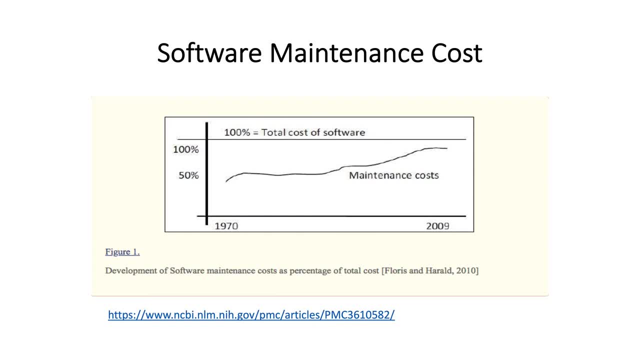 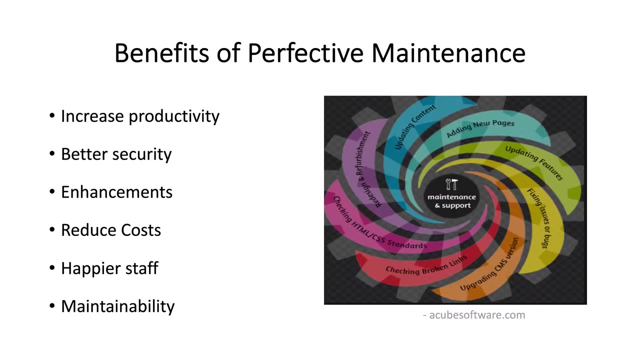 add up to the total cost of software And, based on estimation, the maintenance phase makes up about 60% of the cost. What are the benefits of perfected maintenance? Well, there are multiple benefits that can be observed: Increased productivity, For instance, where software is faster to use. 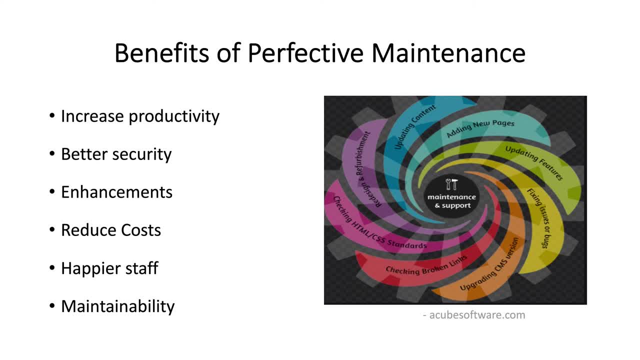 Better security That forces developers to check and validate inputs in a software product. Enhancements, Adding new features that could give competitive advantage In reducing cost. most older software cause issues And, in the long run, incur a cost. Upgrading the software could reduce costs in the long term, not to mention happier staff. 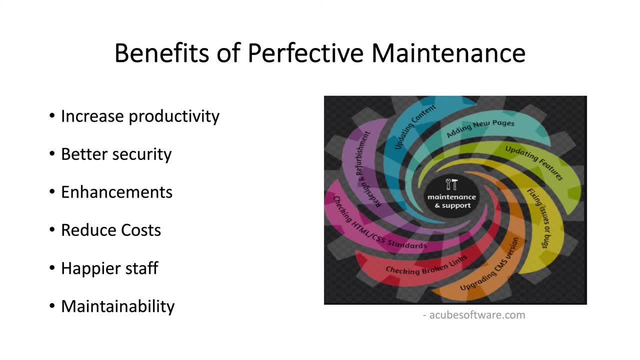 Employees will be able to work more efficiently, And a very important benefit is maintainability, which allows the software to be compatible with the new software and updates. Upgrading the software could reduce costs in the long term, not to mention happier staff, And this is a great way to help developers. 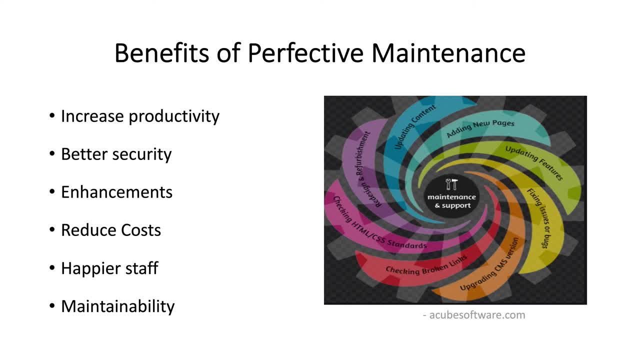 It's an important stepping stone for both a developer and a consultant. However, if you don't know anything yet, please let us know with a comment. If you want to support any of our content, please check the links below And again let us know in the comments section below.